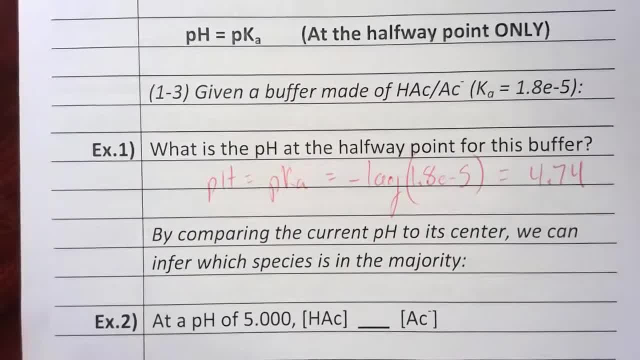 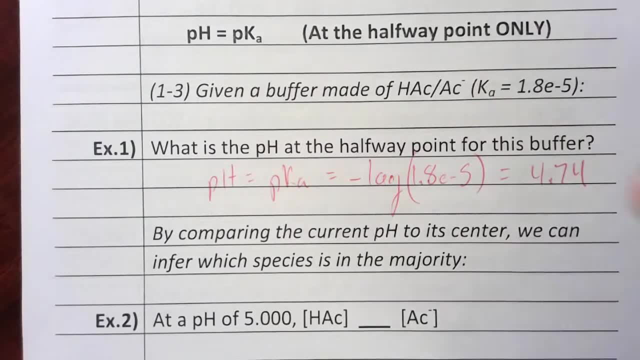 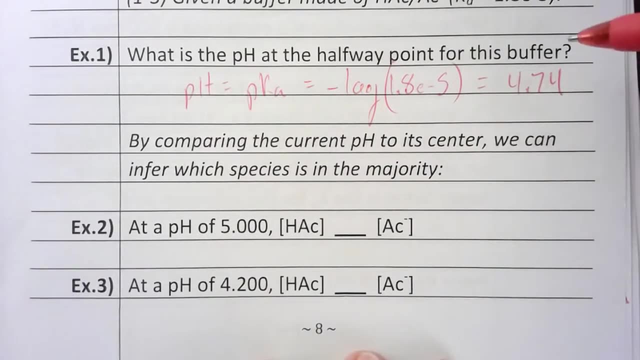 So when a buffer made of HAc and Ac- is at its midpoint, its halfway point, its pH will be 4.74.. So here's what we can do. We can kind of make some comparisons. If you remember, buffers can shift a little up, a little down, depending on the ratio of the Ac- to the HAc. 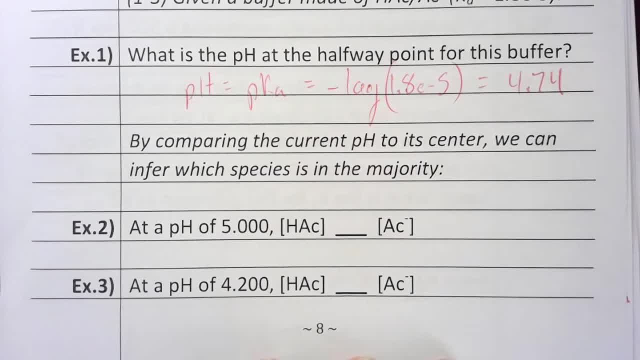 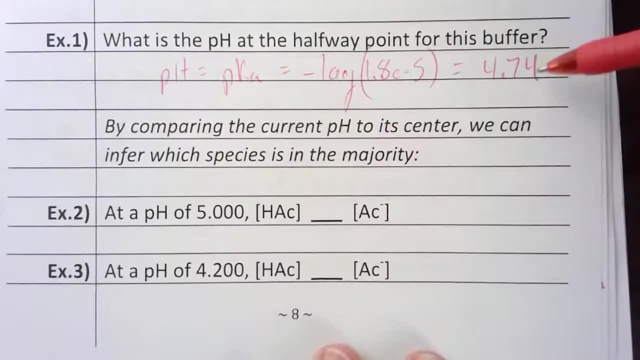 You all remember the Henderson-Hasselbalch equation. Okay, well, pH equals pKa plus log A over HA. The A over HA, The A over HA term is what shifts this either up or down. The higher A is, this is going to shift up. 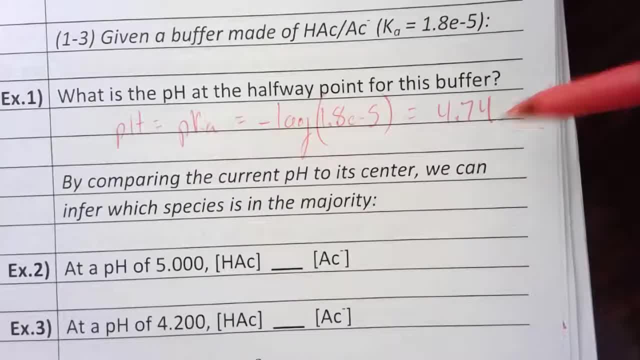 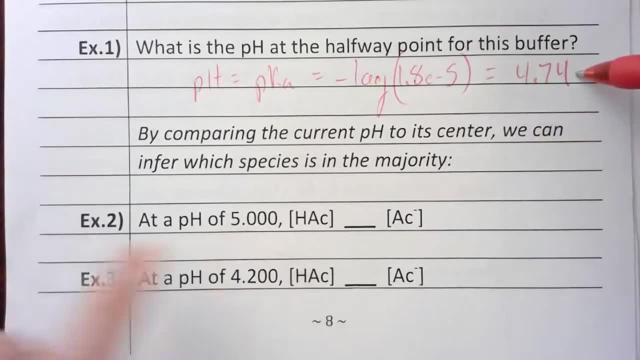 The higher HA is, this is going to shift a little bit down. So let's say that our buffer, the one we're studying here, is centered at 4.74.. Let's say, I give you that same buffer, but it's not at a pH of 4.74,, it's at a pH of 5.. 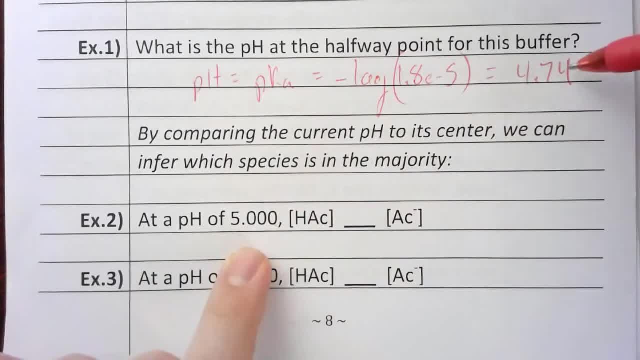 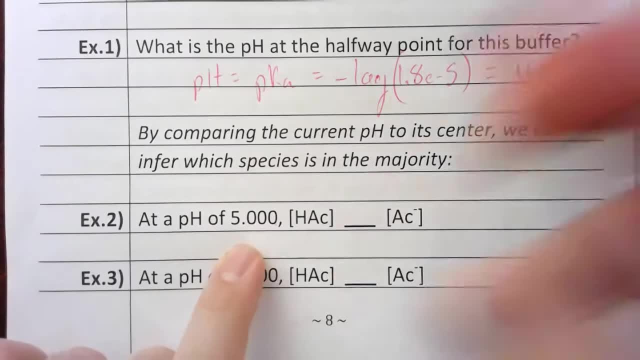 Here's what we know. We know that when the HAc and the Ac- are equal, that it's pH. So the pH will be this. The fact that the pH is higher tells me that the base is winning. So the concentration of the base is going to be a little higher than the concentration. 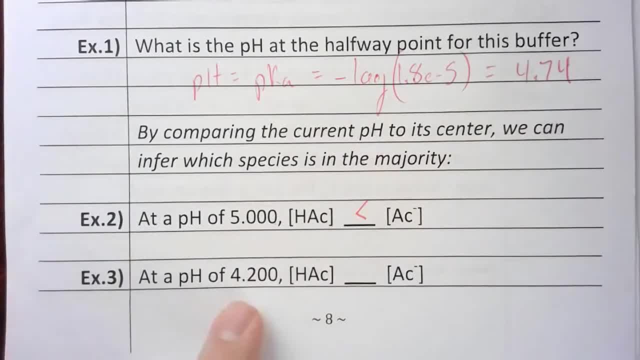 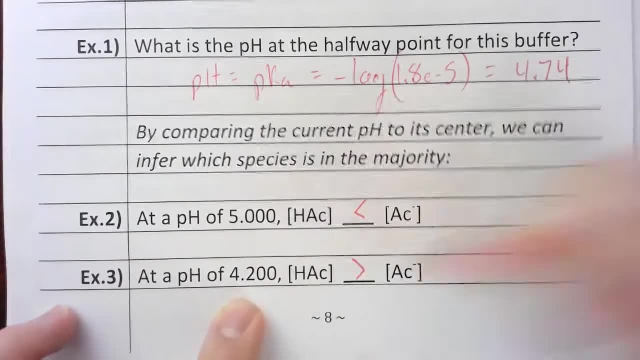 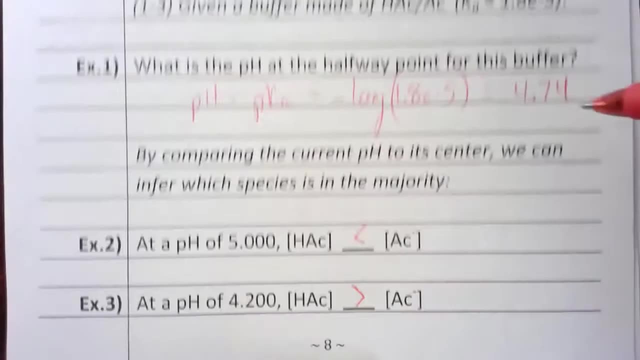 of the acid in this buffer And then at a pH of 4.2, the opposite would be true. This is a little lower than the midpoint. therefore there must be a little more acid in it than there is base, And this is what is meant by the buffer shifting up and down just a little bit around its midpoint. 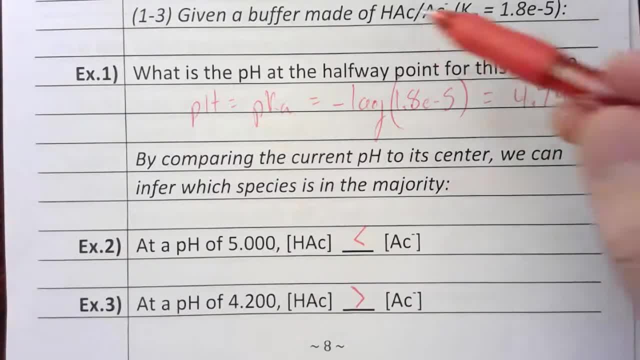 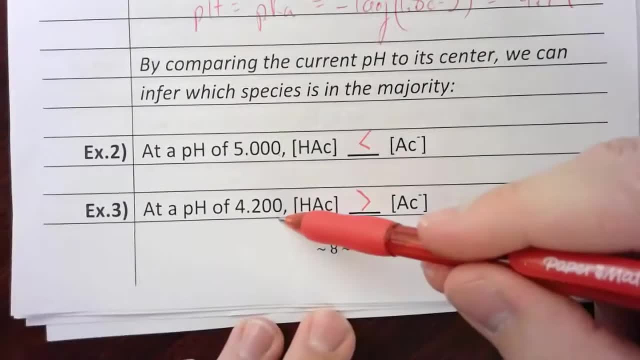 So, again, This is where the buffer A equals HA or, in this case, HAc equals Ac- If the HAc is a little higher, the pH goes down. If the Ac- is a little higher, the pH goes up. 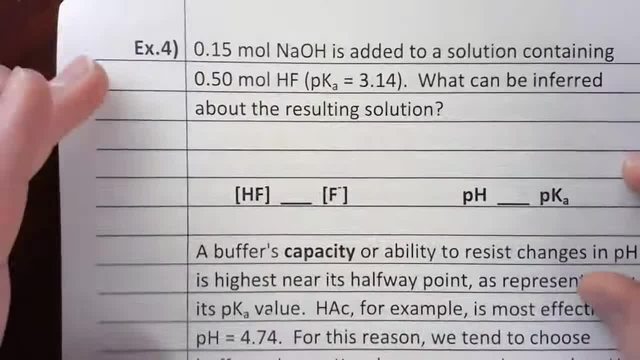 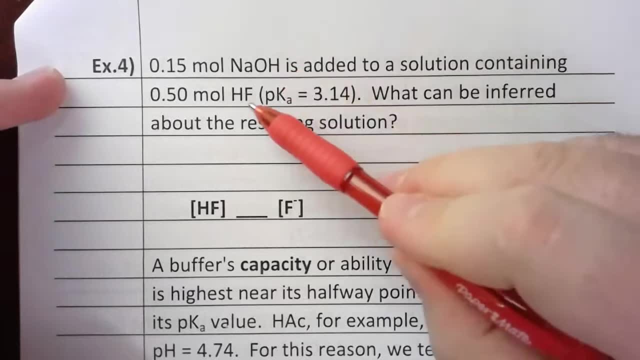 And that's all there is to it. So number 4 is a little tricky. Okay, keep in mind. this strong base is going to convert some of the HF into F- I want you to go ahead and figure out which of these two would survive. 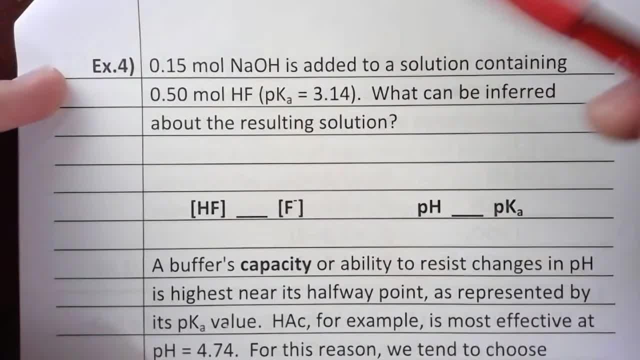 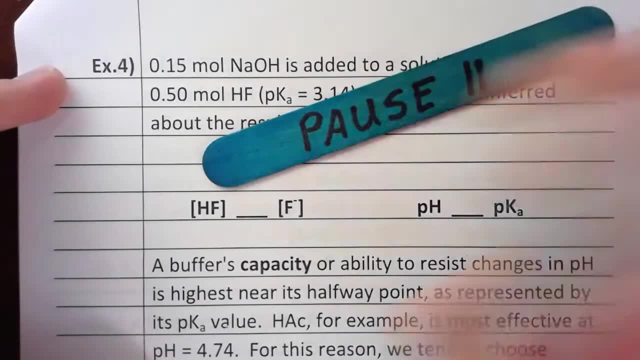 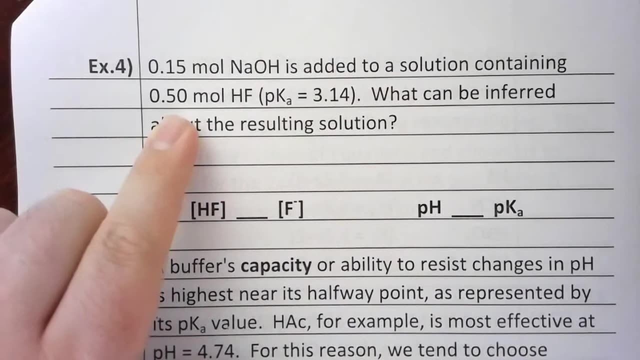 And in what amounts, And what will happen to the stuff that is made? Based on that information, you should be able to answer this question. Give it a shot. So the NaOH is going to completely react with the HF. The HF will survive because it's in excess. 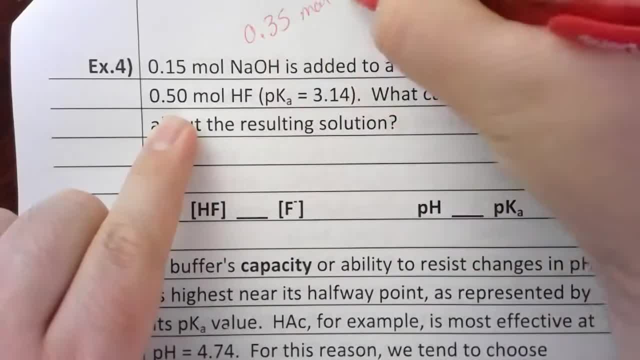 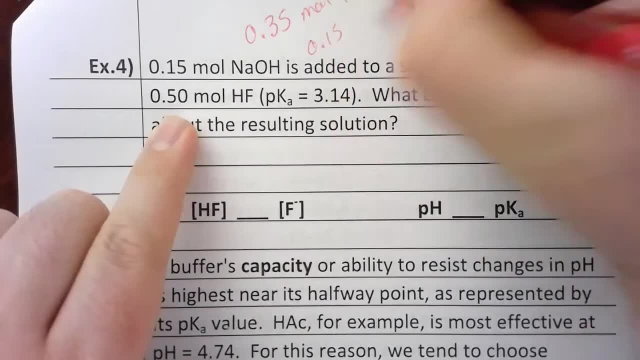 Only 0.35 moles of the HF will survive. All the remaining HF, all the HF that went away, is going to become F-, and that would be 0.15 moles. Okay, So the HF is going to be 0.15 moles of F- when this is all said and done, 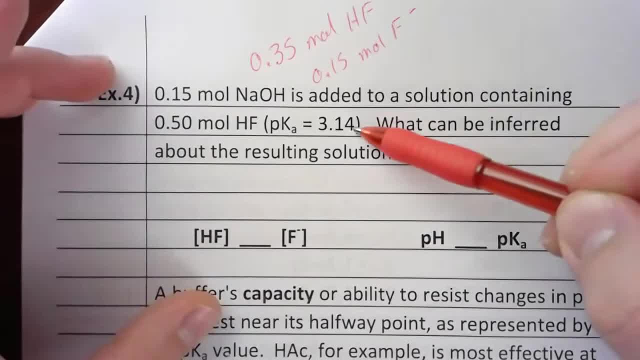 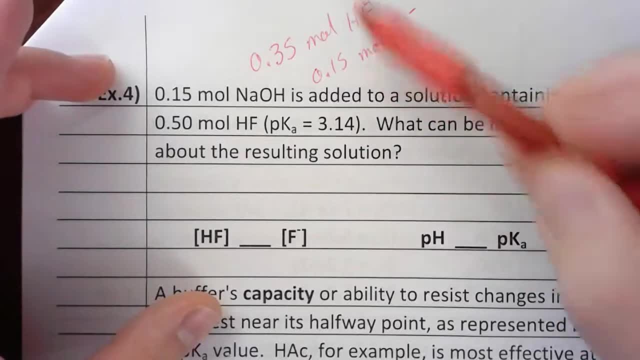 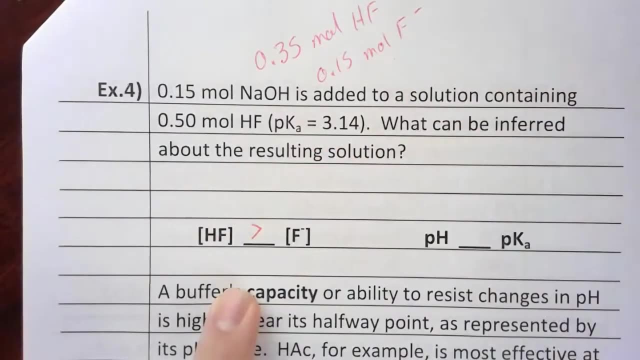 So here's what I know. I know that this is the midpoint of this buffer. The pH will equal this. when these two are equal, Well, I'll tell you what they're not equal. So I know that the HF- just by looking at this, I know the HF is going to be higher. 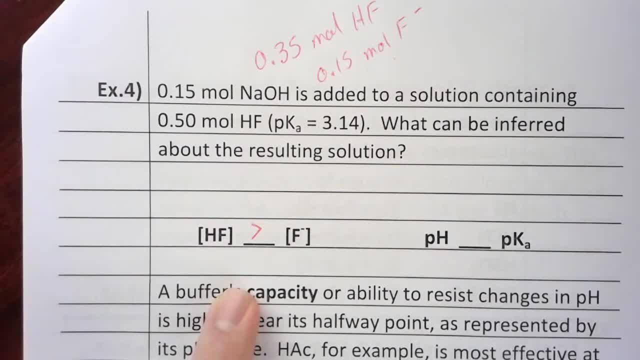 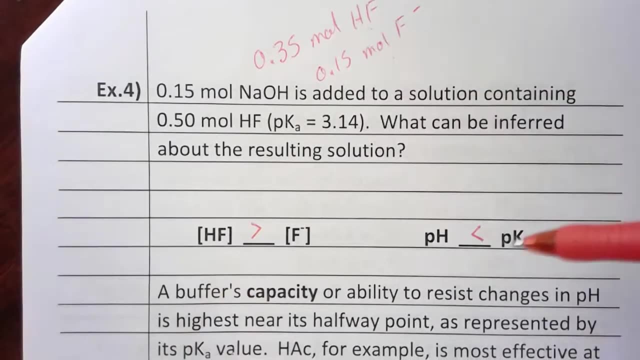 than the F. What effect will that have on the buffer? Well, it'll drive it down a little bit. The HF is an acid, So the pH will actually be less than the midpoint, because the midpoint's a 50-50.. And when the HF is winning, the pH is going to be a little lower than we expect, because 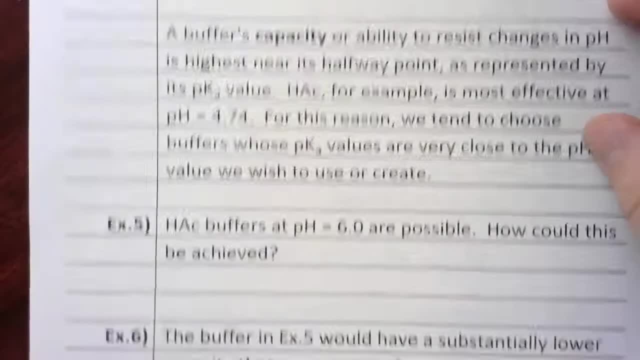 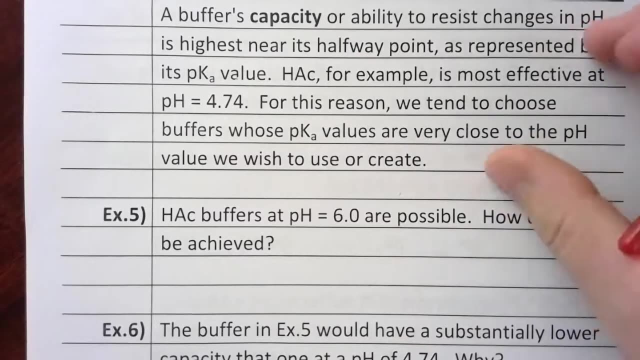 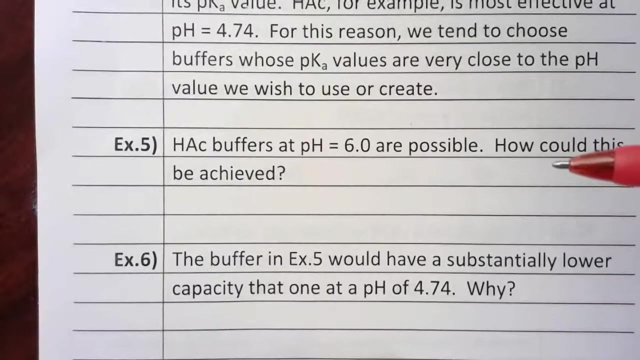 the HF is an acid, All right, So try reading this, And these two are concept questions. I want you to take a shot at five as soon as you're done reading this, See if you can figure it out. Okay, So it's possible to get a decent range out of a buffer, even one that's centered around. 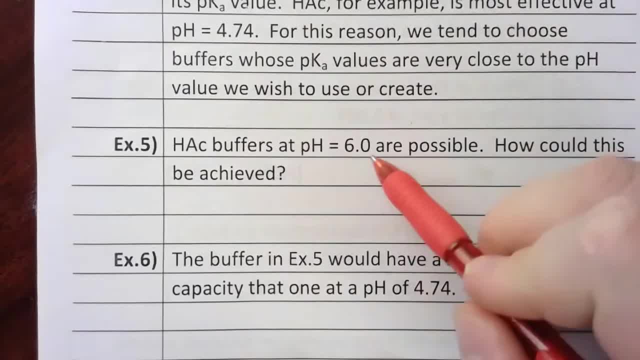 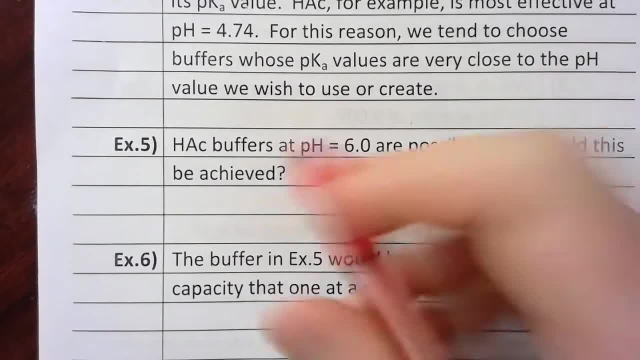 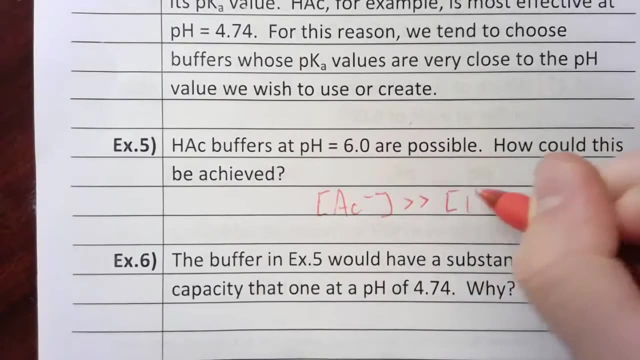 4.74.. If you wanted a buffer containing a pH of 6.0, you would have to push the base pretty high. So the only way to do this is to make it so that the concentration of AC- is significantly higher than the concentration of HAC. 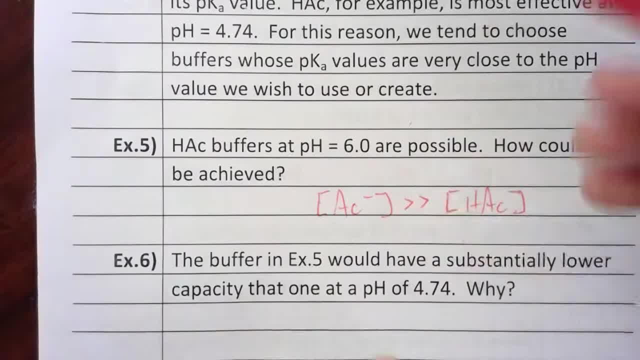 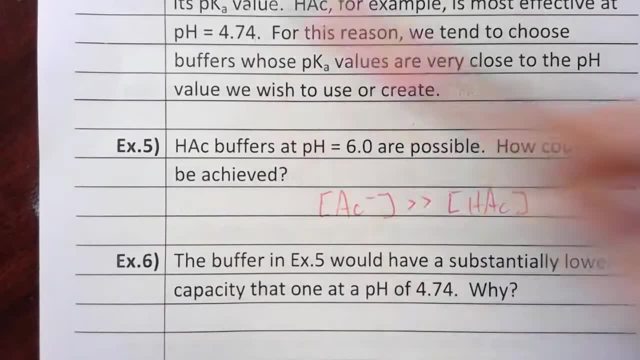 Basically, you're pushing the buffer's pH Okay Above its center point because, remember, these two would be equal at 4.74.. In order for the pH to be substantially higher, the AC- must be the majority by a pretty substantial. 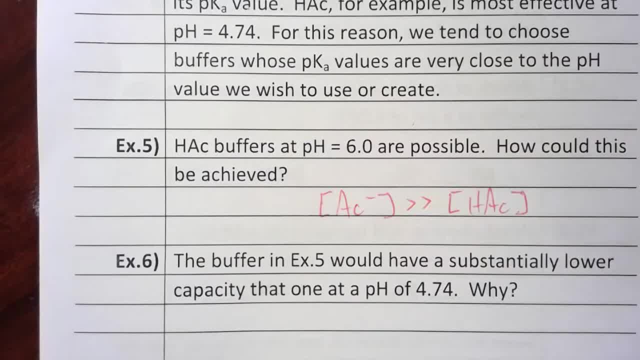 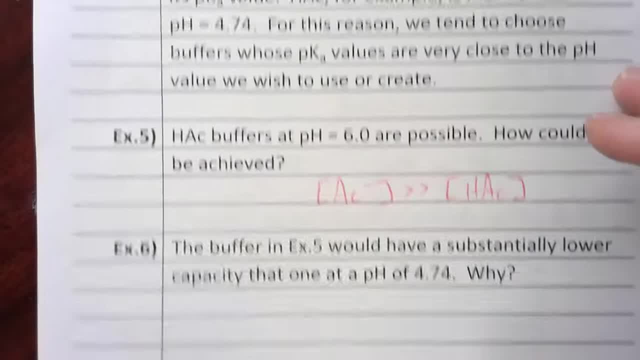 quantity. Now there is one slight problem. This buffer isn't going to be able to take much abuse. It's not going to be able to buffer for very much longer. I want you to try and speculate. why would this buffer be so ineffective at 6.0 than? 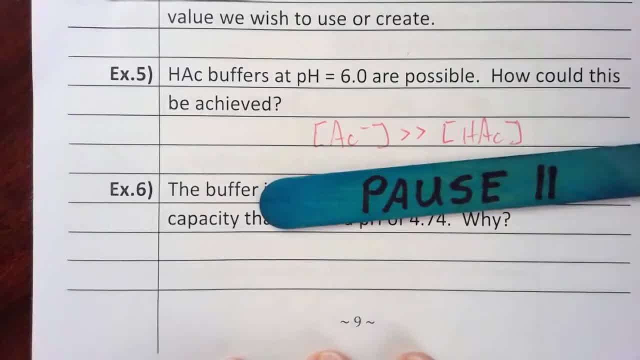 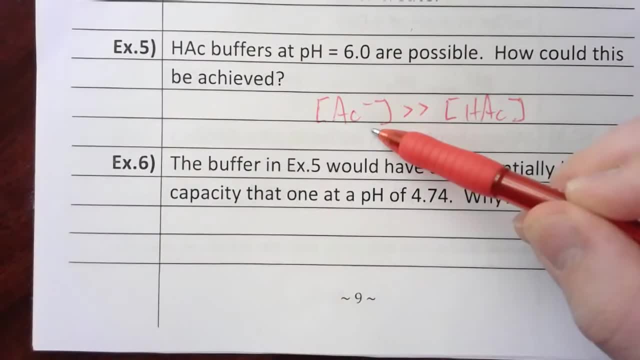 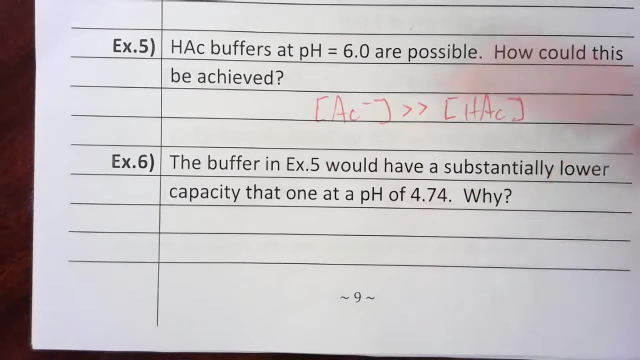 it would at 4.74.. Take a shot at this, Okay, Because there's so much more AC-. this buffer is going to be very effective at handling acids because there's a lot of AC- and that's what will react with the acids. 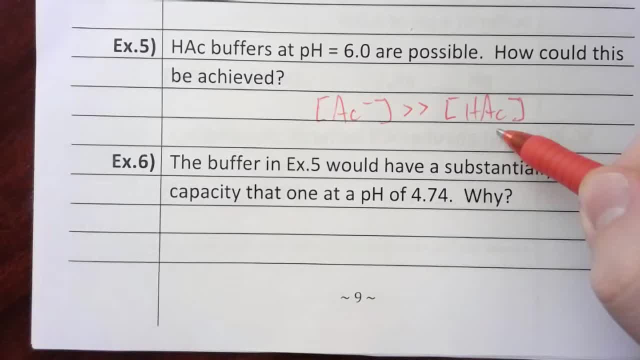 But there's very little HAC left. so while it is still a buffer, there's not a lot of the weak acid, which means it's not going to have a very high capacity for handling bases. So the very low concentration of HAC is going to be very effective at handling acids. 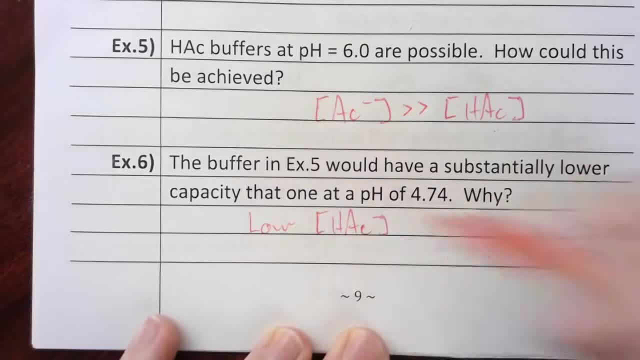 So there's very little HAC left. Okay, So the very low concentration of HAC greatly decreases capacity for strong. what, Take a guess, guys, The HAC? what would it react with? It would react with the strong bases. 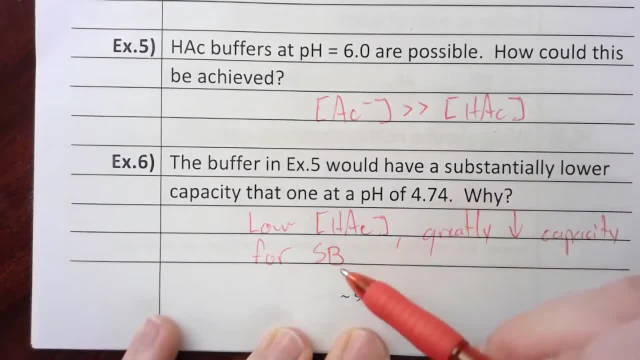 This buffer can't handle the addition of a strong base because there's very little acid left. So there's a good chance. this buffer's already been pushed. What's the difference? already been pushed very close to its collapsing or breaking point. there's a very good chance. 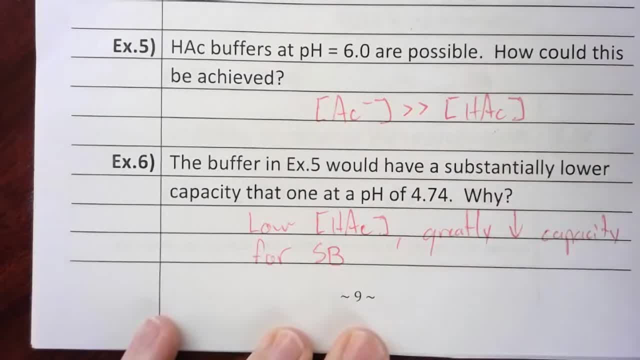 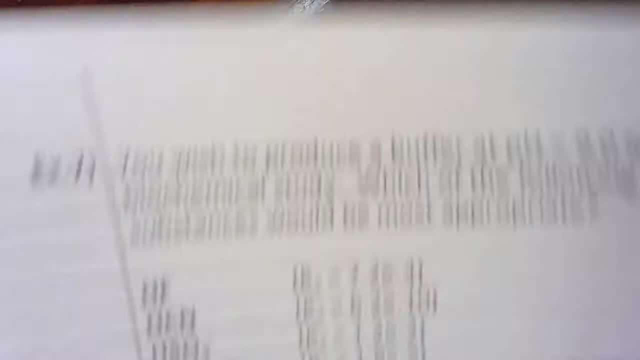 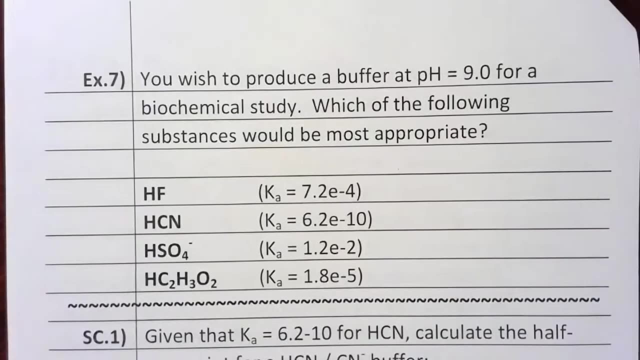 that a single drop of a strong base would cause the buffer to collapse, because there wouldn't be any more HAC left, And that's how it works. Now one final thing: If you choose a buffer, you choose a buffer whose center point is very close, the halfway point. 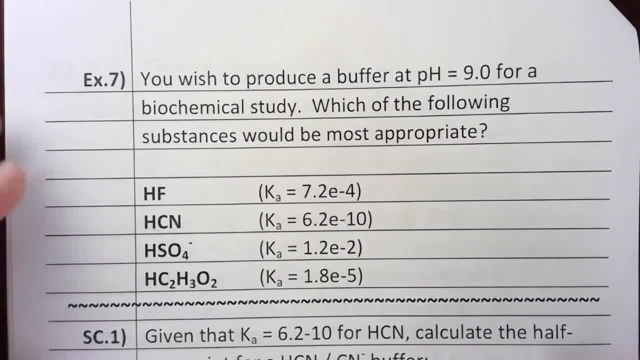 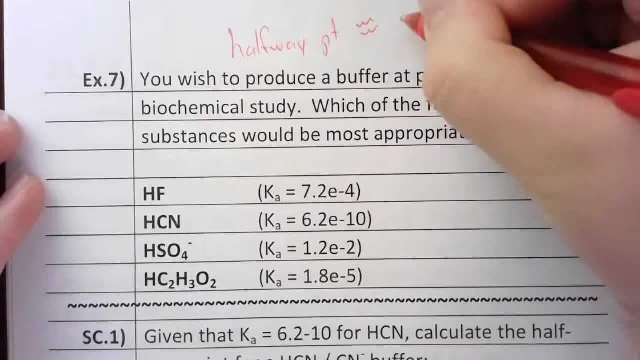 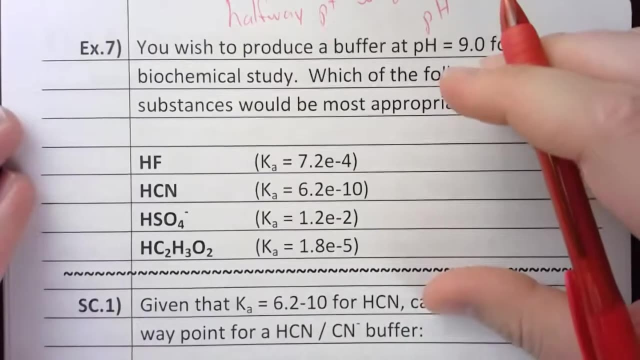 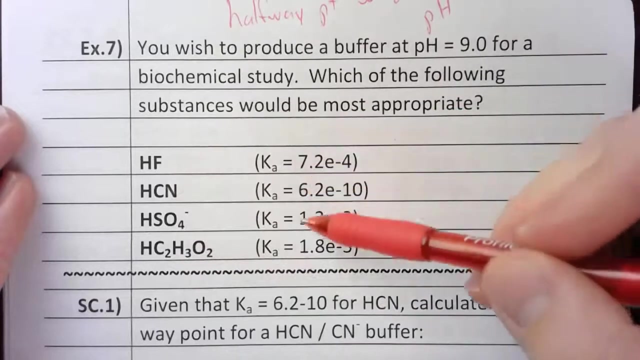 is very close to the pH you want. So you want the halfway point to be approximately equal to the desired pH. Now I've given you a series of buffers, each of which are a series of weak acids with which you could make a buffer, And I've given you Ka values for each. 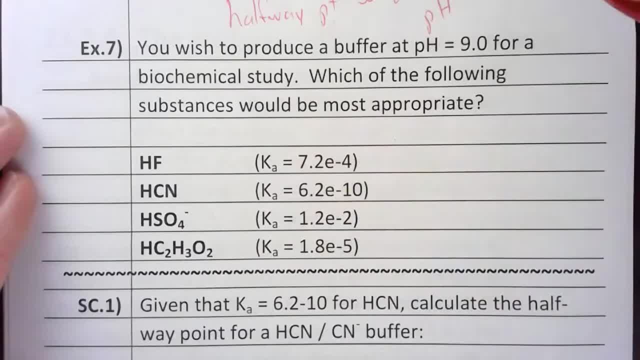 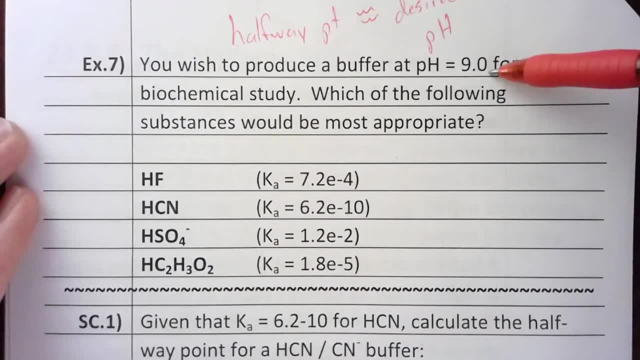 of them. I want you to tell me which of these substances would be most likely to cause the decrease in pH and which of these substances would be the most likely to cause the decrease in pH and which of these substances would be the most likely to cause the decrease in.